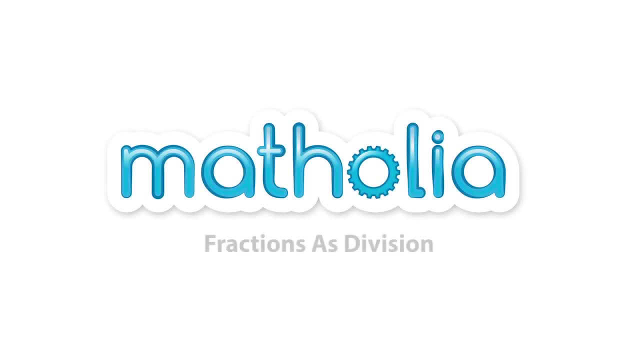 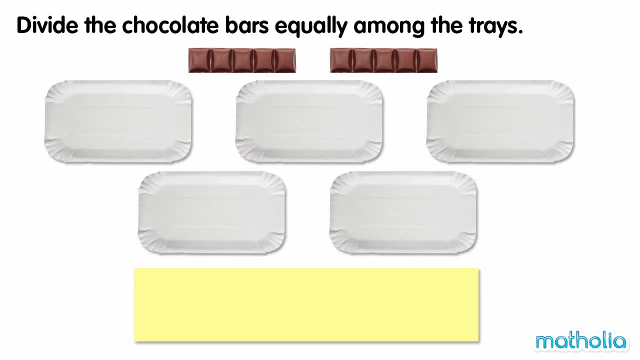 Divide the chocolate bars equally among the trays. There are two chocolate bars and five trays. We need to find two, divide five. Each chocolate bar is made up of five pieces of chocolate. Let's divide the chocolate among the trays by placing one piece on each tray until we have used up all of the pieces. 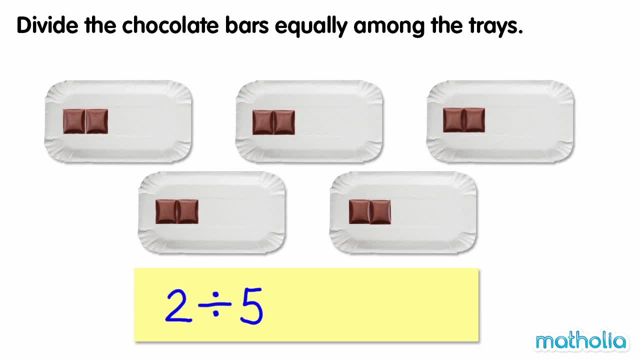 We have divided the two chocolate bars equally among the trays. Each tray contains two fifths of a bar of chocolate, So two divided by five is equal to two fifths. When dividing two whole numbers, the quotient can be expressed as a fraction that has a numerator equal to the dividend and a denominator equal to the divisor. 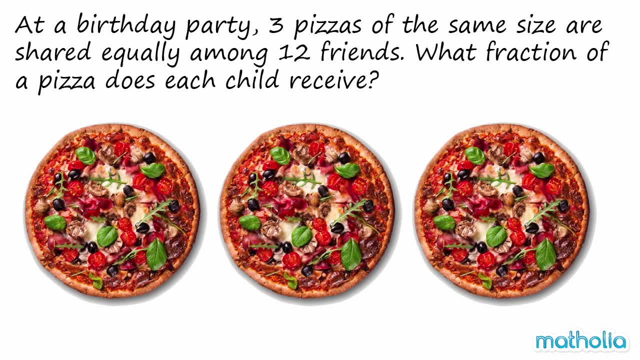 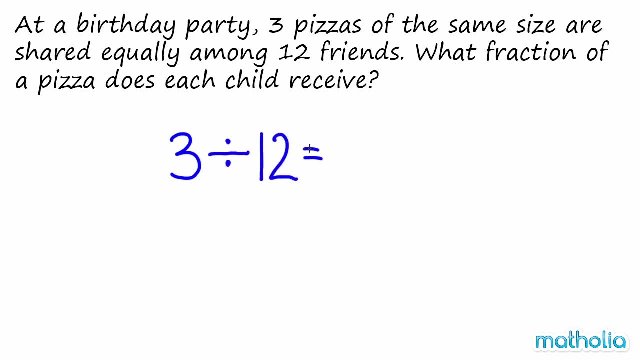 At a birthday party, three pizzas of the same size are shared equally among twelve friends. What fraction of a pizza does each child receive? We need to divide the number of pizzas by the number of children. Three divided by twelve is equal to three fifths. 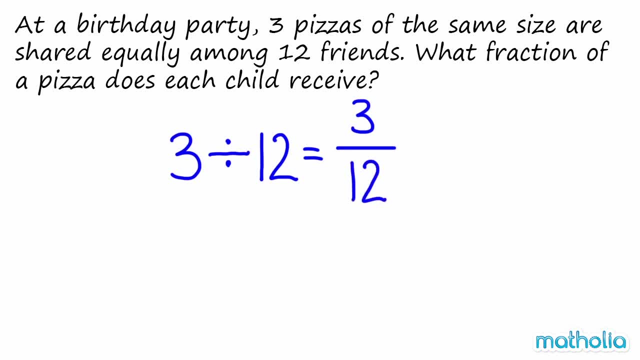 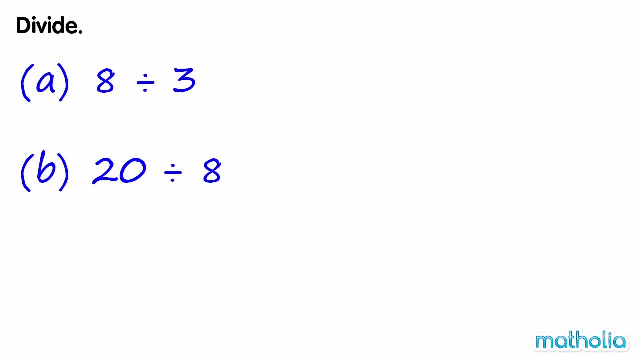 We can simplify three twelfths by dividing the numerator and denominator by three to give one quarter, So each child receives one quarter of a pizza. Divide Eight divided by three is equal to eight thirds. Eight thirds is an improper fraction which we can express as the mixed number two and two thirds. 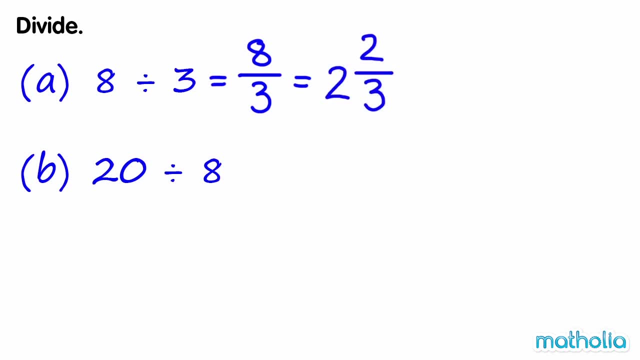 So eight divided by three is equal to two and two thirds. Twenty divided by eight is equal to twenty eighths. This is also an improper fraction That can be expressed as the mixed number two and four eighths. Four eighths can be simplified to one half. 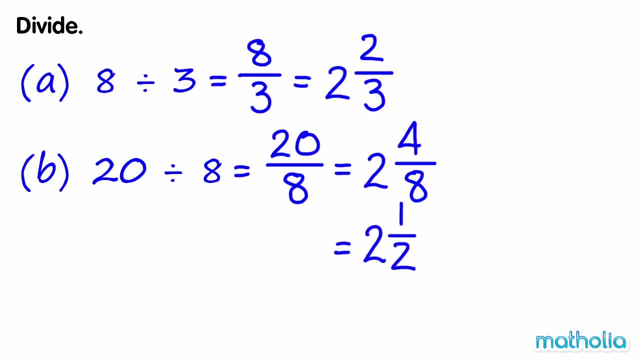 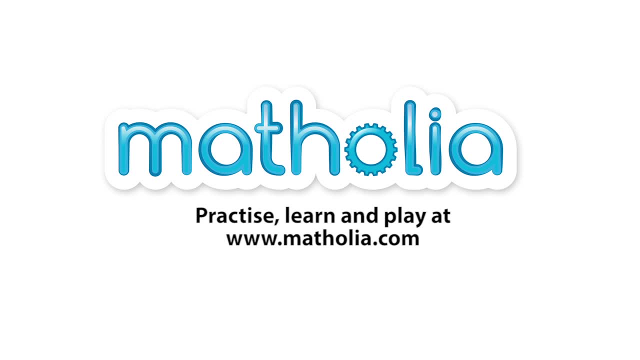 So twenty divided by eight is equal to two and a half- And we can see the uniform Robin Hood's card as forward in the message here- And four over paar eighths would bearemos a pop stimulus. The next two rhizomes might be like three and a half in number. two and two eighths would be like two thirds, and two lovers would be like five eighths. So to put the quotient professional between two and two eighths.